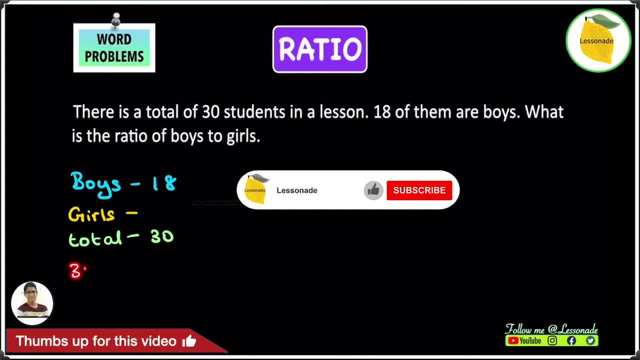 and the number of boys. so that means we have to do 30 minus 18, which will give us 12. means the number of girls is 12.. so now we have found out the number of boys and girls. next we have to write these in a ratio. so the ratio is boys to girls, because we're doing from boys to 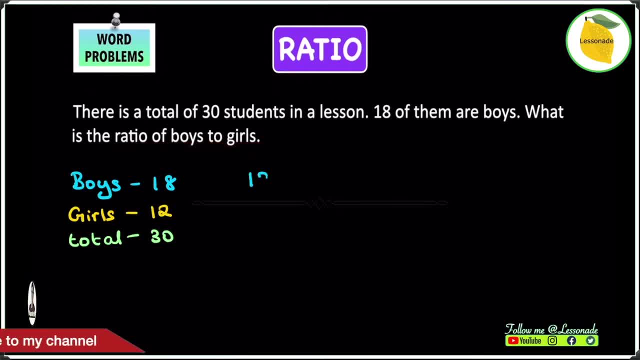 girls. we need to write the boys first, which is 18, and then the number of girls is 12.. so we're getting a ratio of 18 to 12.. now we can simplify 18 to 12.. to do that, we need to find the highest. 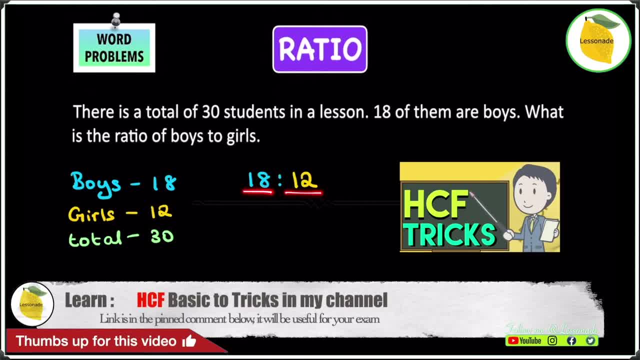 common factor for both girls and girls. so we need to find the highest common factor for both girls- 18 and 12.. if you guys want to know how to find the highest common factor, i've got a video on that. the link is in the description below, so go check that out. so we have to find the highest common. 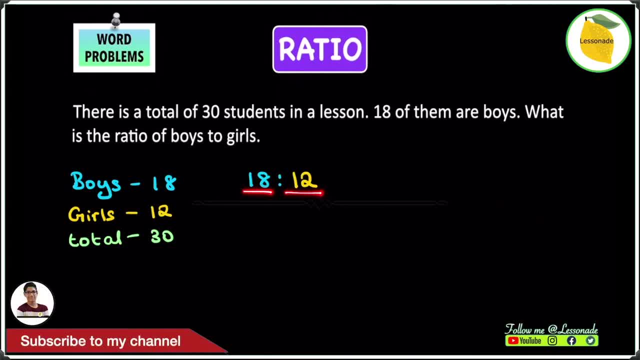 factor. the highest common factor of 18 and 12 is obviously 6, which means we have to divide with 18 and 12 by 6.. so 18 divided by 6 will give us 3, and then 12 divided by 6 will give us. 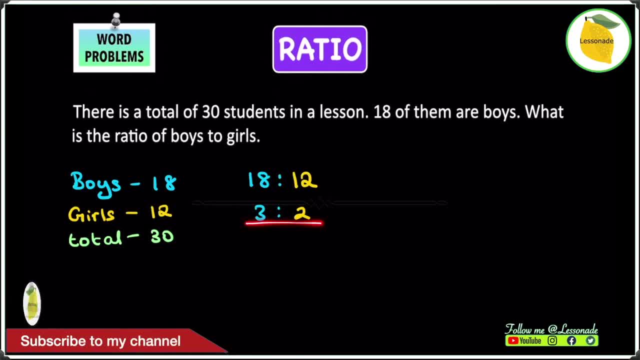 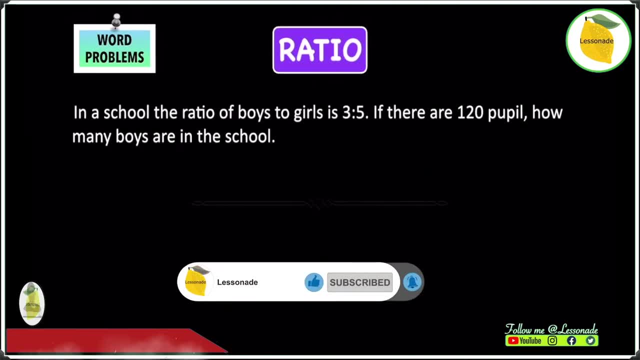 2, which means we get an answer of 3 to 2 and therefore our ratio to this question is 3 to 2.. now let's have a look at another example, and in this example it says: in a school, the ratio of boys to girls is 3 to 5.. if there are 120 people, how many boys are in the school? so, as you guys, 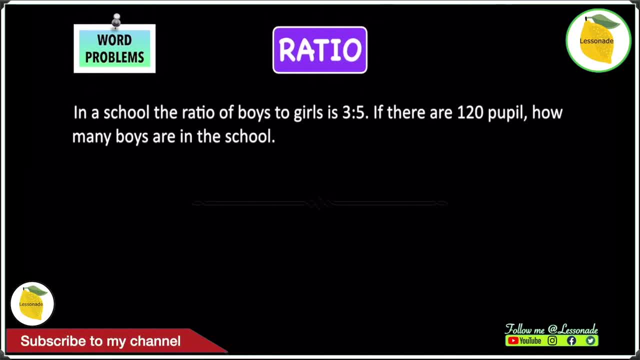 could see. in this question this is a bit different to the one we looked previously, because in the first one we had to find the ratio. instead, in this question we have the ratio. we have to find the number of boys in the school. so, firstly, let's write boys and girls down, because we need to. 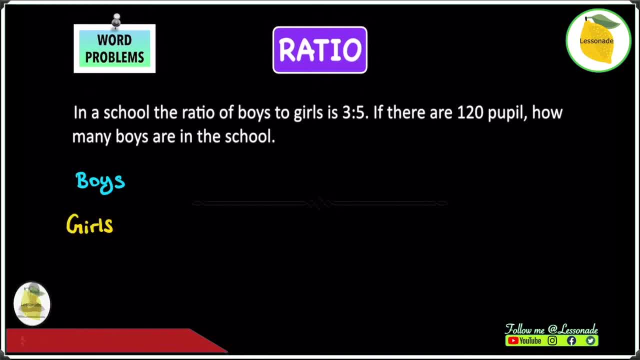 find both of these first, so the boys and the girls. so now, as you guys could see, we go back to the ratio. it says 3 to 5. so 3 to 5 is the ratio for boys to girls. so for the sake of this question,